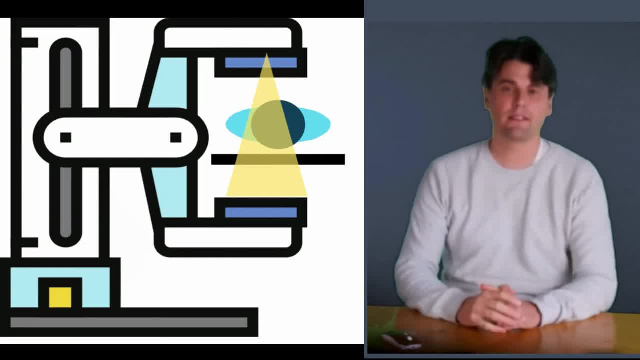 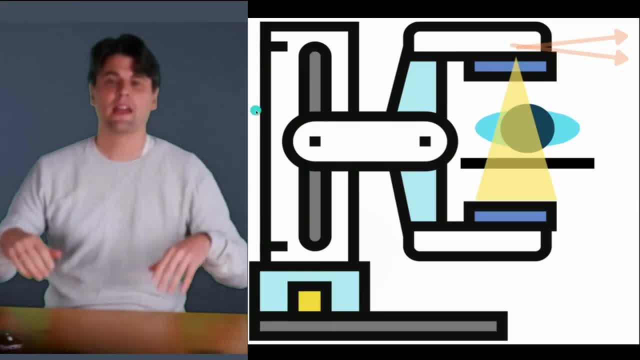 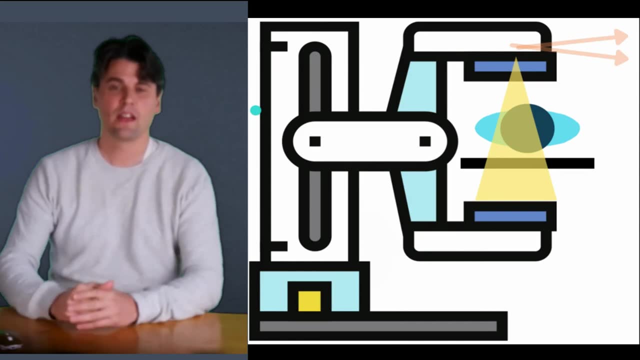 be generating our images directly, definitely want to minimize the time that you're going to spend with any appendages within the direct beam. second area, then, of radiation within the room is potential scatter from the housing itself of the x-ray tube within the process. it's what's. 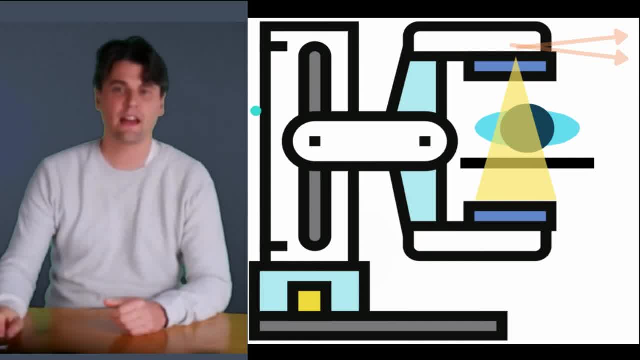 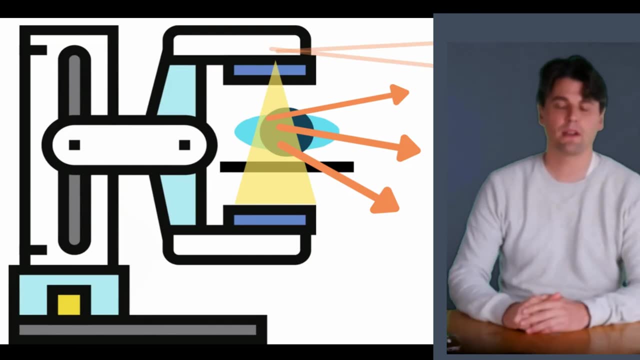 called all focal radiation and scatter from the x-ray tube within the x-ray tube itself. this leads to a relatively low background radiation within the room. the third area, which is actually the one that we're trying to minimize our exposure, is actually scatter from the patient themselves. 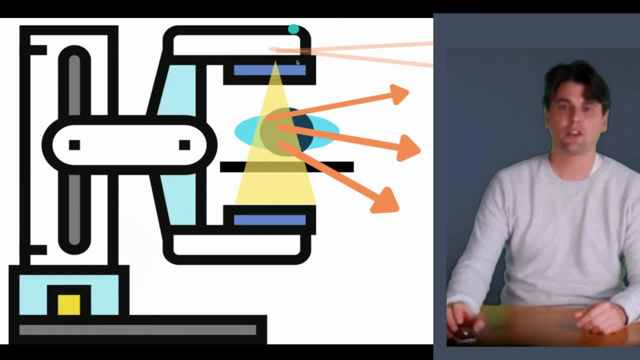 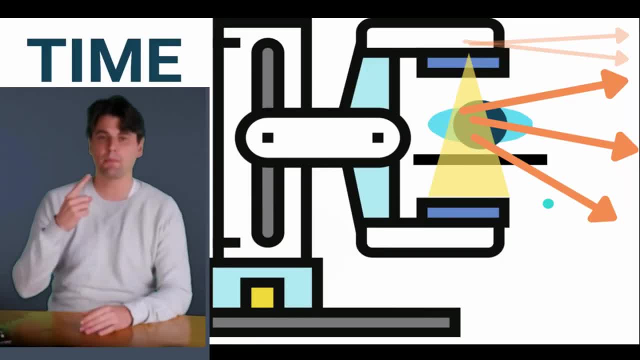 x-rays again are interacting within the patient and you're going to have compton scatter coming out all throughout the room. time we want to, number one: minimize the time the x-rays are on and minimize the time that the staff is in the room when the x-rays are on. if we minimize the time that the 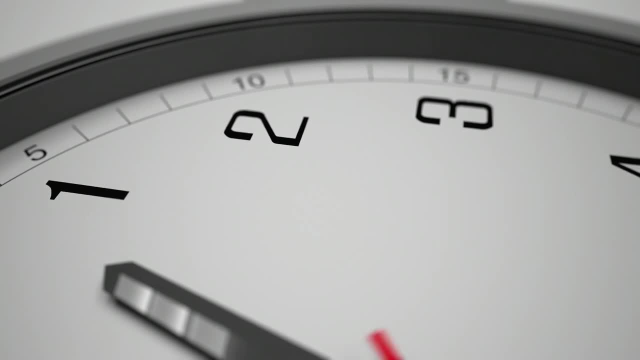 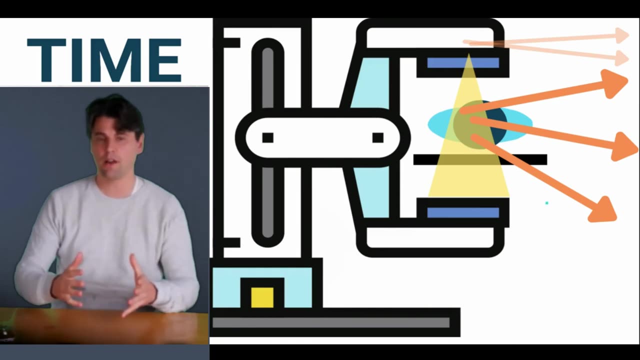 x-rays are on, that's going to minimize our exposure to the x-ray tube within the room- secondary radiation. this is a direct relationship because right after the x-rays are turned off will not be additional radiation within the room. this is our second tool in order to minimize the 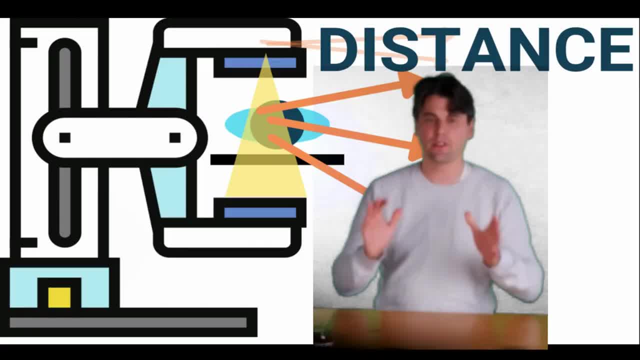 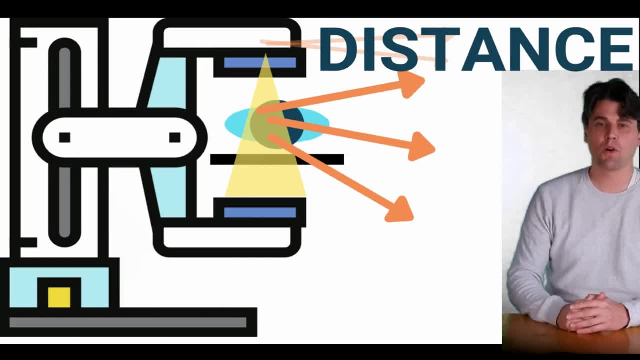 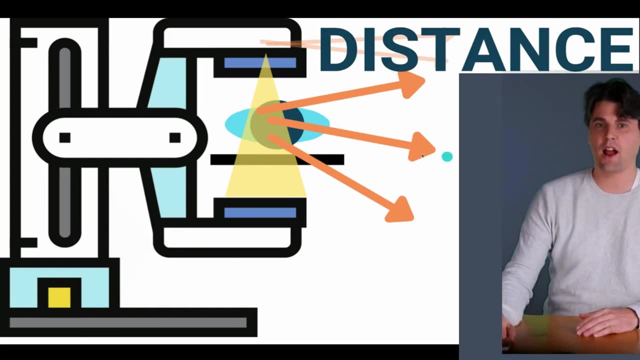 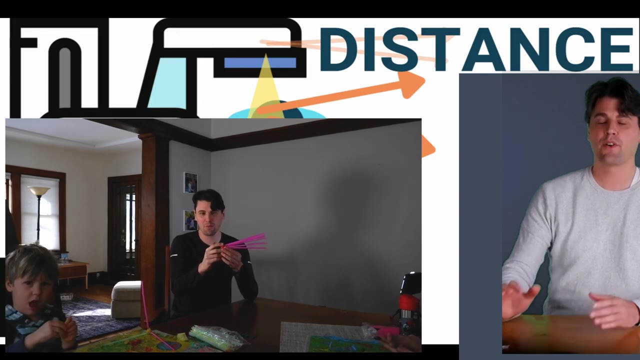 radiation exposure that we have. so if we start at this distance, move to this distance, we can see that there's going to actually be a lower radiation exposure. this has to do with the one over r squared principle, because you can see, our x-rays are actually diverging or actually traveling apart or moving away from one another. so the further you are, 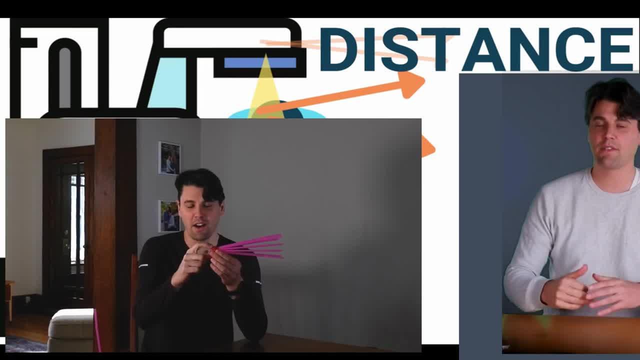 the lower intensity of x-rays you're going to have. you can check out our video on the one over r squared. if you move two times further away, you will then only have one quarter of the x-ray intensity shielding. shielding is also a very important tool in the tool kit. 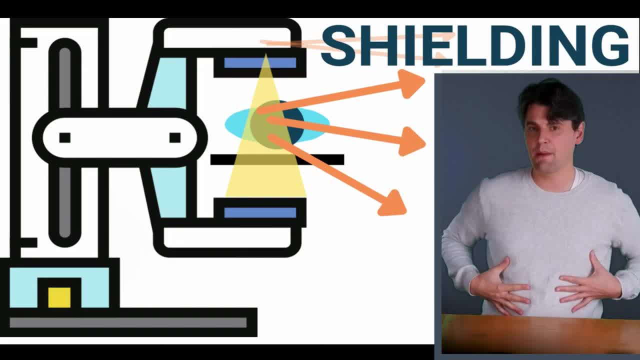 there's a variety of shields you can have, including lead aprons which can be worn, and including translucent lead impregnated materials such that you can have additional photoelectric effect to your advantage with that lead. because it's a hy-z material, it's going to be efficient.